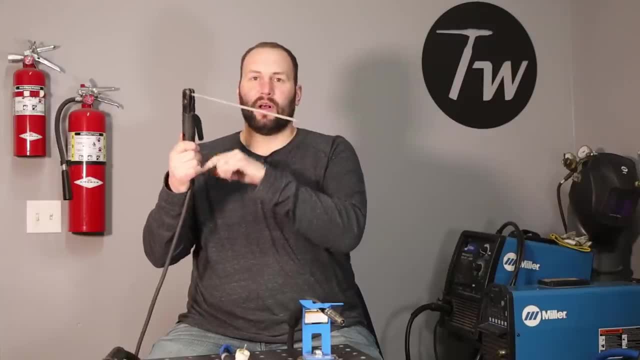 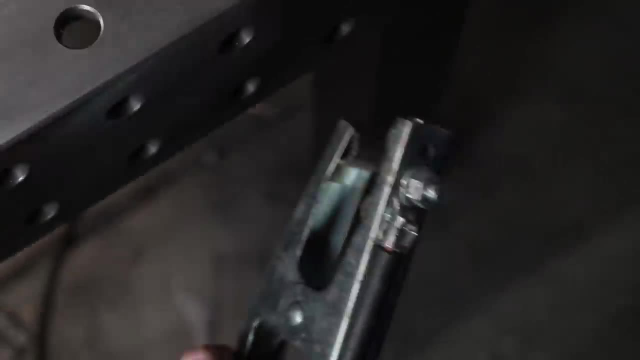 it And that allows electricity to flow from my welder up through the rod, And then I'll put this other clamp on my welding table or you can put it on the part you're working on to complete a weld And then I'll connect it to that rod there And that makes a short circuit and will create a. 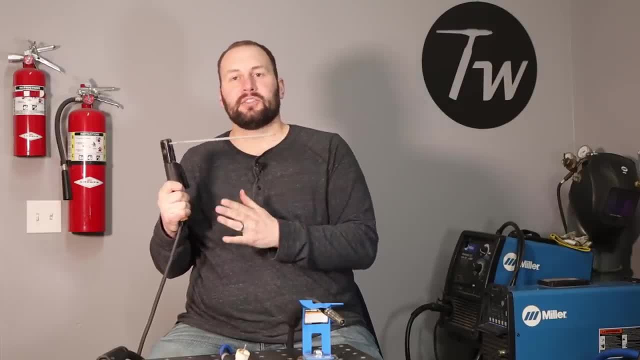 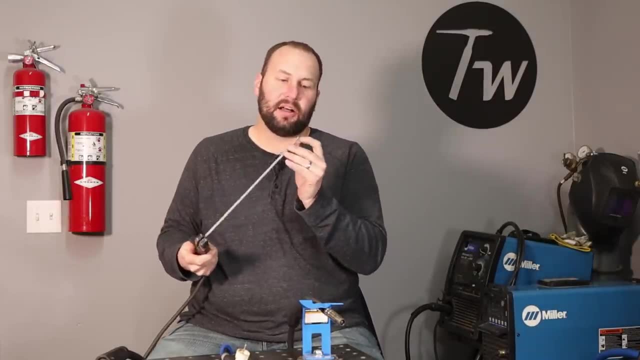 spark that starts an arc, And the arc is where electricity jumps over a gap and creates a tremendous amount of heat. Now, when that happens, it melts your base metal and it also melts off the center of this rod and adds it to it. That's why you get that crowned up shape on your weld. 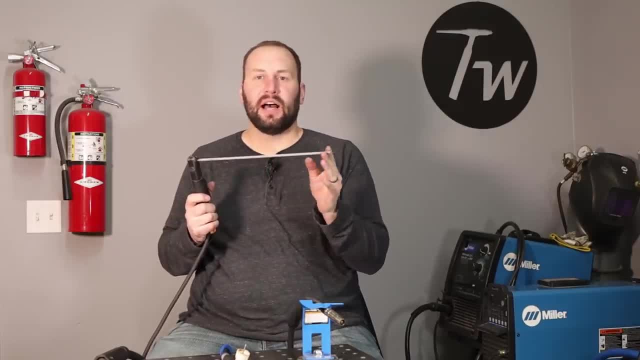 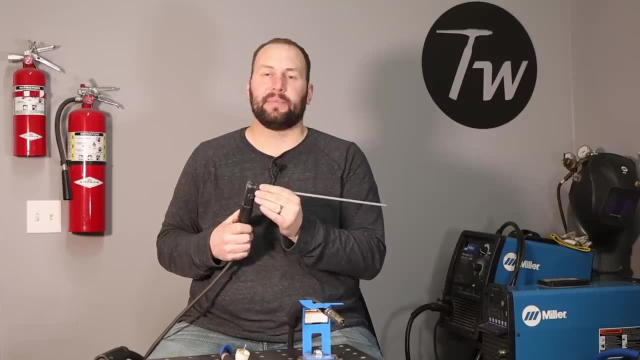 The other thing that happens is this outside coating that's called flux burns off and it protects that molten metal from the air so that it doesn't get burned, And that's why you get that contaminated by oxygen and other things in the air. So it's really genius how that works. 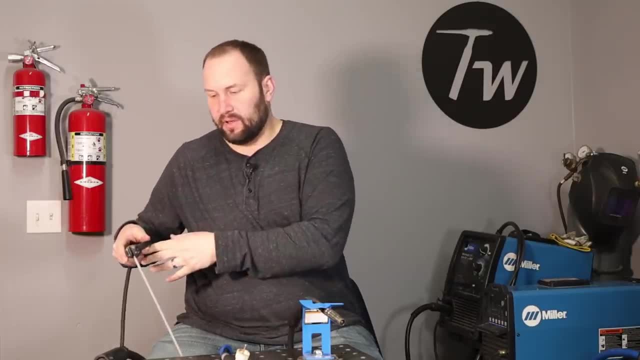 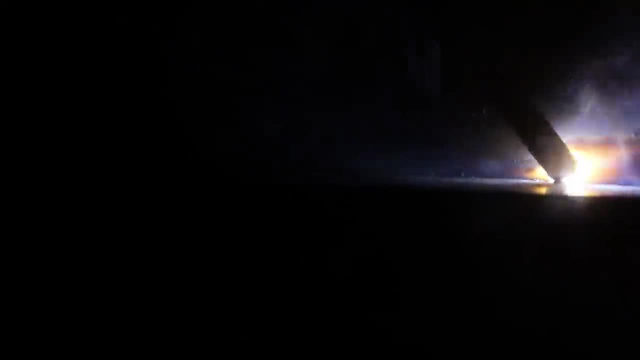 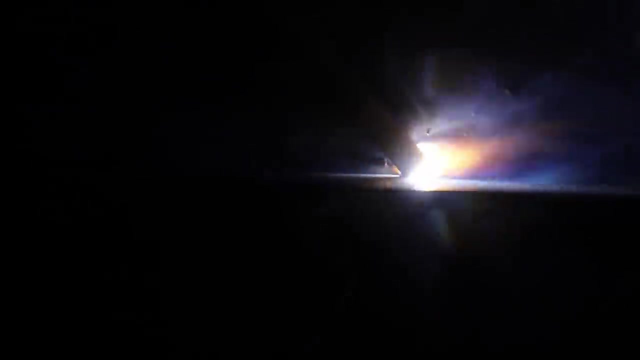 Now, as you move along, your rod will burn down from long to short. And let's go ahead and do a little demo So you can see as I'm welding here, the electrode is just maintaining that nice short arc, And that's because I'm moving my hand in closer to the metal as I move along, And it's 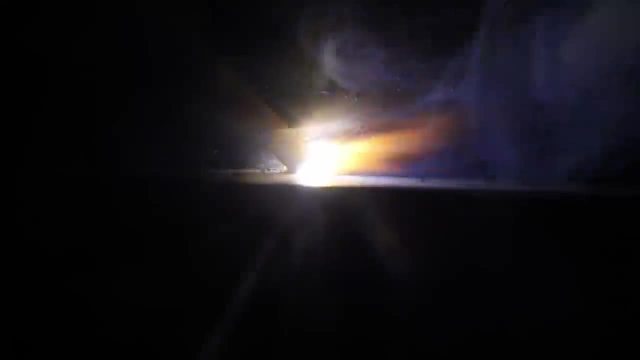 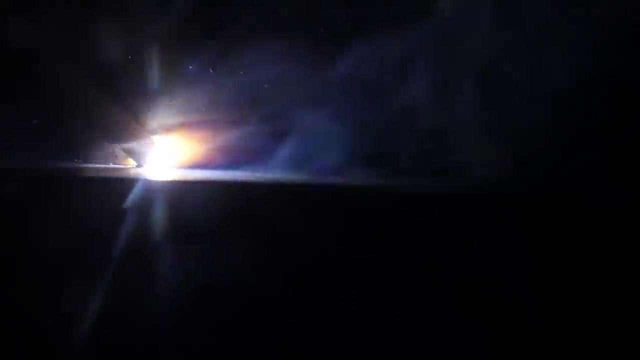 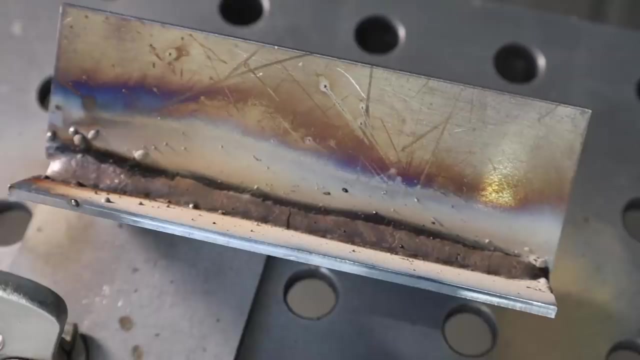 just, you've got that bright spot where it's really hot. It's depositing that metal in and it's also burning off that flux and leaving a coating on the top of the weld called slag. Now at the end of the weld here you can see that slag coating remaining. And I'll go ahead and just 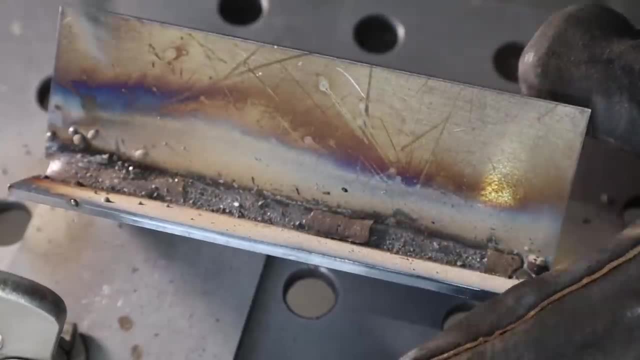 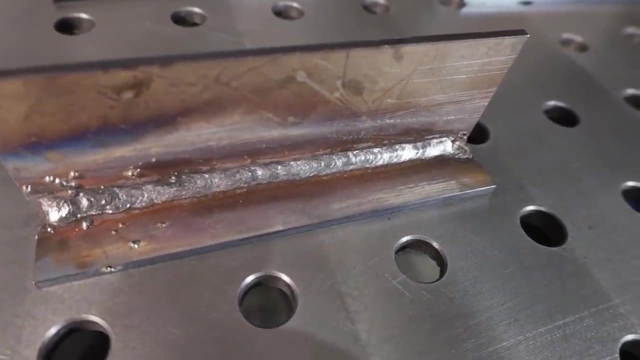 remove it with a tool called a chipping hammer, And after I rake that off and clean it up, you can see I have a nice result. So stick welding is really good for a few reasons. One: the equipment is inexpensive. So if you're going to do a lot of work, you're going to want to make sure that you 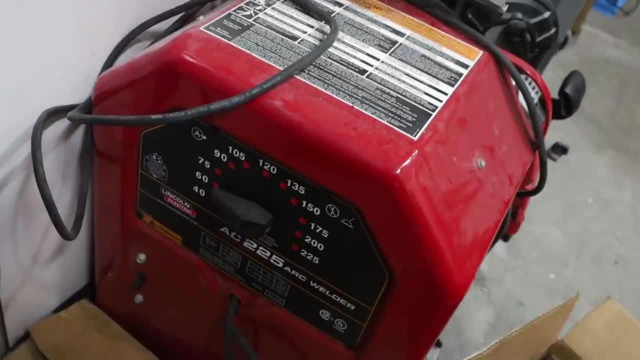 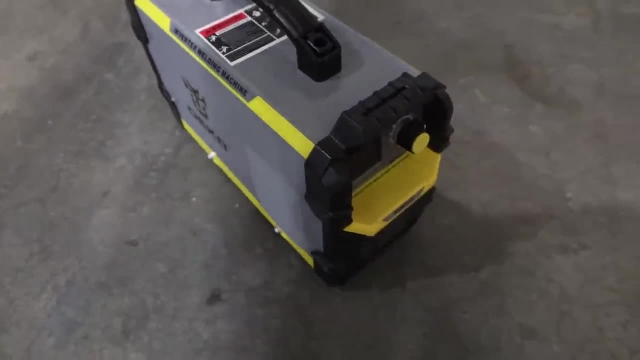 you can have a basic arc welder like this Lincoln tombstone buzz box, or this is another stick welder that I picked up for about a hundred dollars on Amazon. that works pretty well also, And so it's very portable, very simple. You just need one of these and some rods, along with your. 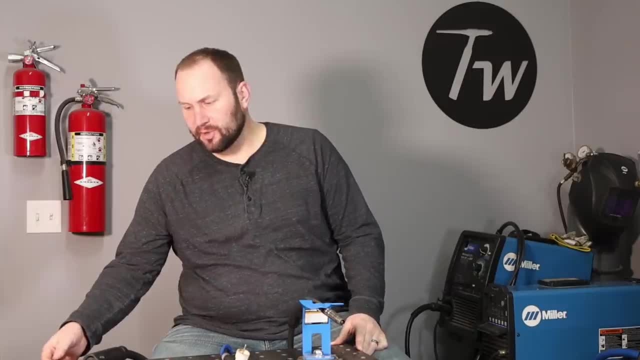 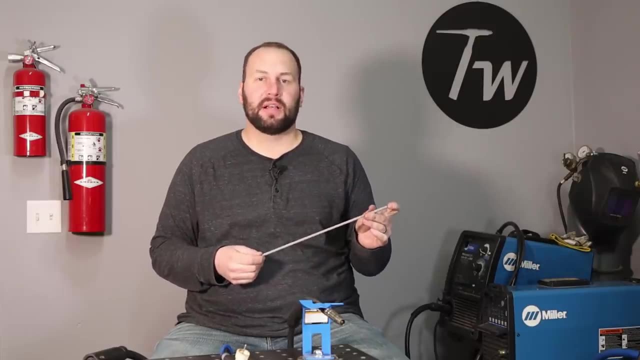 safety gear and you're basically in business. You're ready to go. Some of the drawbacks are that slag coating that it leaves, So I wouldn't use it for like auto body sheet metal. That will be more of a challenge than other processes. I also typically won't stick weld anything like that. 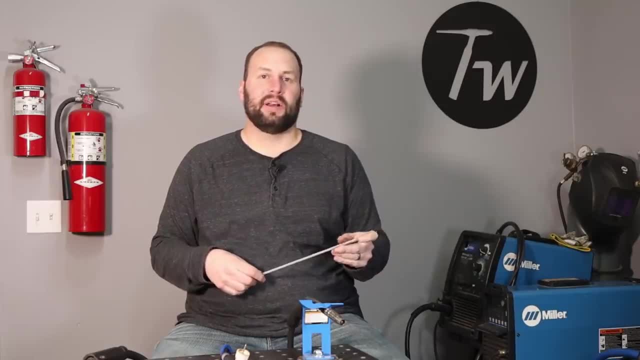 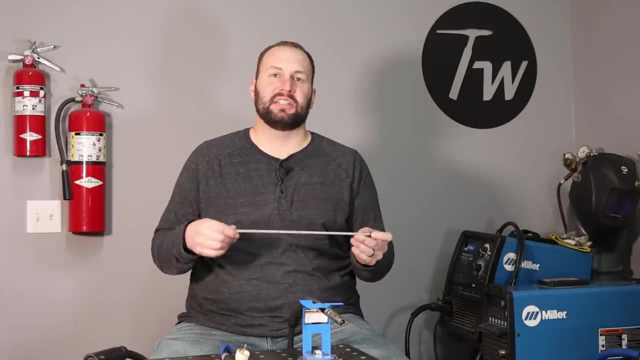 I'm not going to do anything that's thinner than about one 16th of an inch or a one and a half millimeters that you can if you do it right, But I usually try to avoid that because it becomes pretty challenging to avoid burning through. But it's really good for anything that thick or 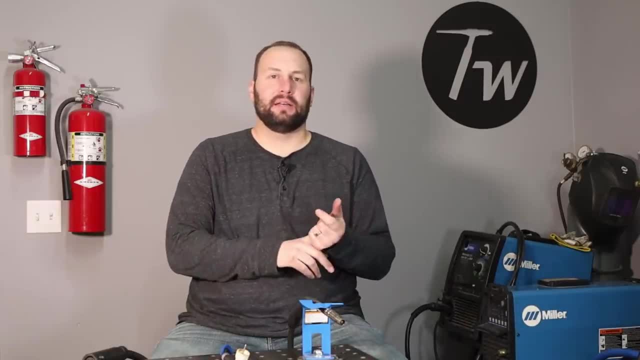 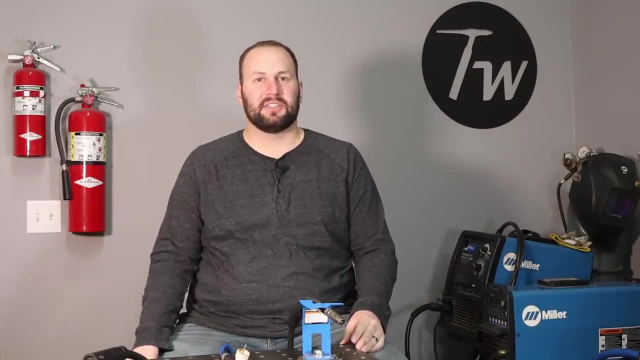 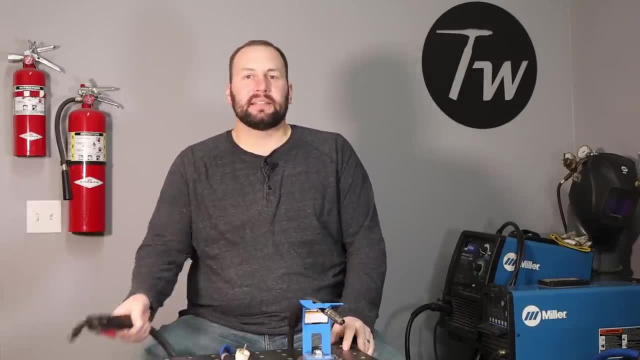 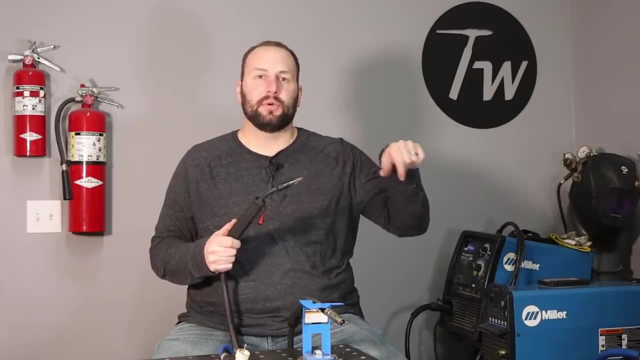 But it's a really good process. It's used a lot in industry still, especially on the pipeline. Next let's talk about flux core welding, And it's basically the same process as stick welding, in that you deposit your metal through an arc and you shield it with the flux. But imagine taking the 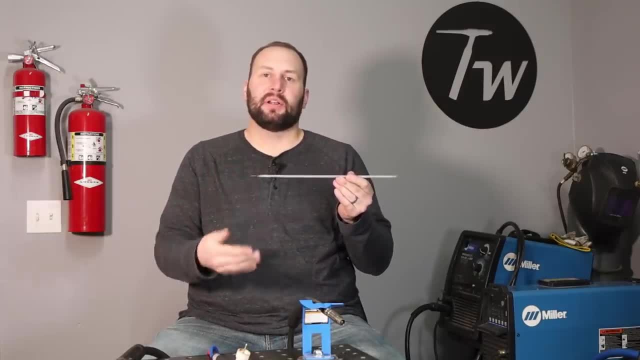 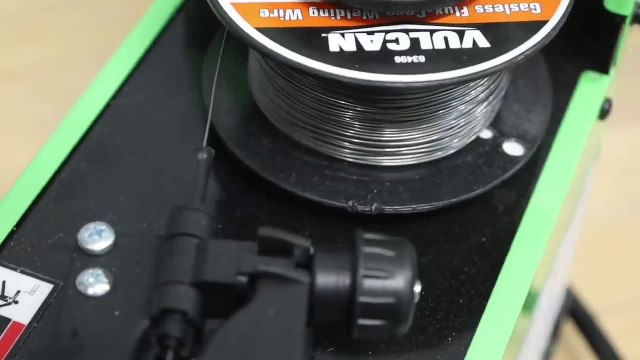 stick welding rod and you turn it inside out, So you take the metal and put it on the outside of the flux and then you wind that around a roll and you feed it with a motor instead of feeding it manually with your hand. And that's what you have here. 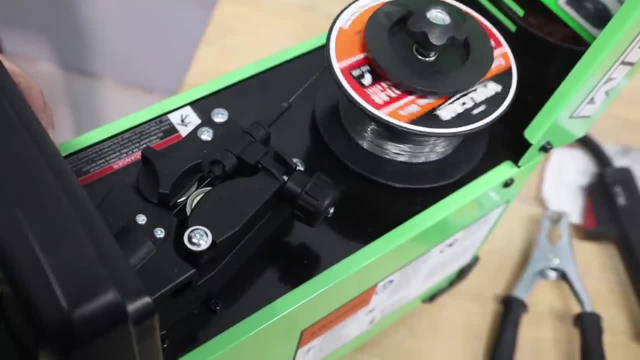 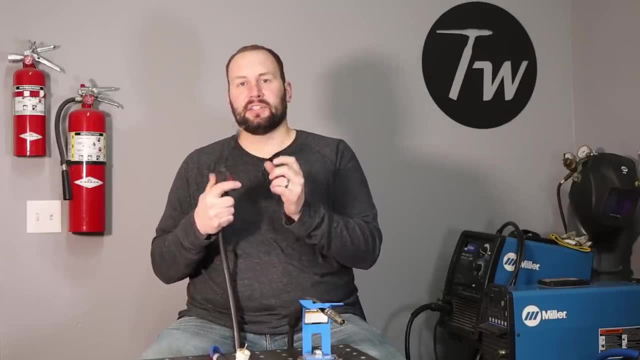 is this feeding mechanism and you push it through a tube and out of gun. Now, some of the advantages here are: one: it's easier because you don't have to worry about striking an arc. It kind of happens on its own when you push the button. 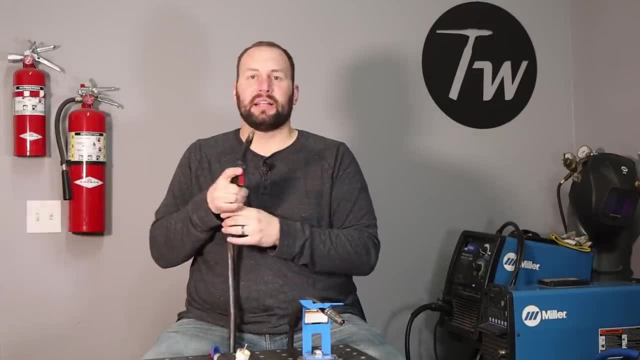 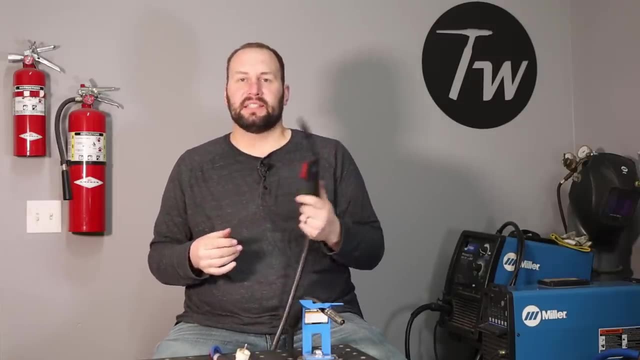 Also, you just maintain the same distance and you don't have to stop when your electrode runs out. So it's definitely much easier than stick welding to learn how to do. It can also be done with relatively inexpensive equipment. This is just on a basic flux core welder from Harbor Freight. 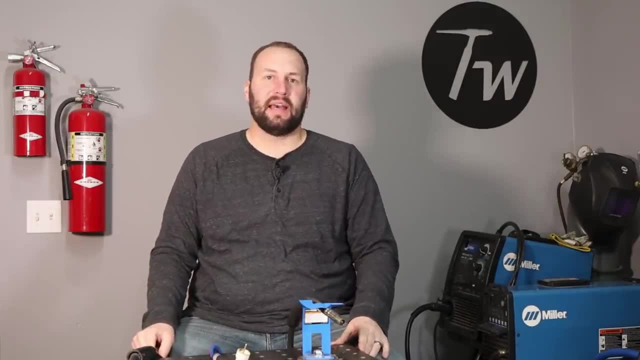 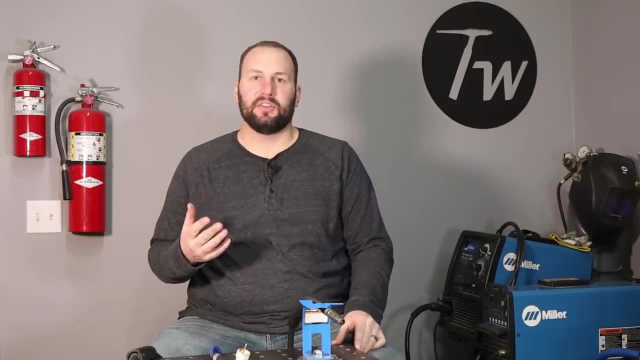 that's less than $200, and there's other similar ones than that. This one I've had for a little while and use it from time to time and it's worked well. Or you can use basically any MIG welder. So if you know you're going to want to, you know, learn to MIG weld one day. 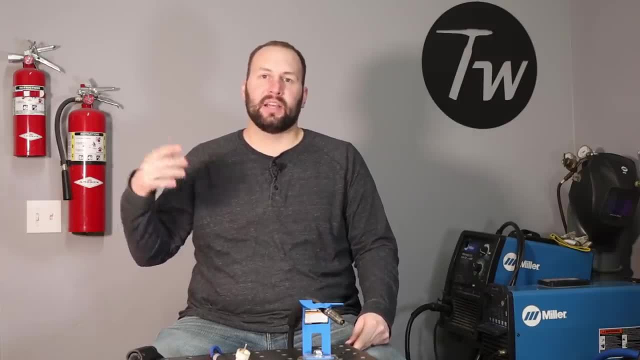 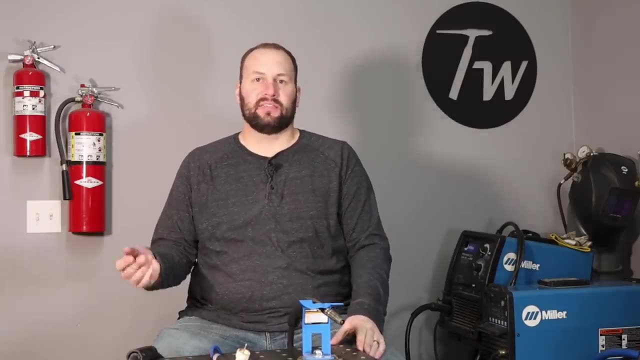 or add the gas cylinder to do that. you can get a MIG welder and set it up for flux core now and then grow into it, So it's really good for that. It can weld, you know, anything from thinner sheet metal. 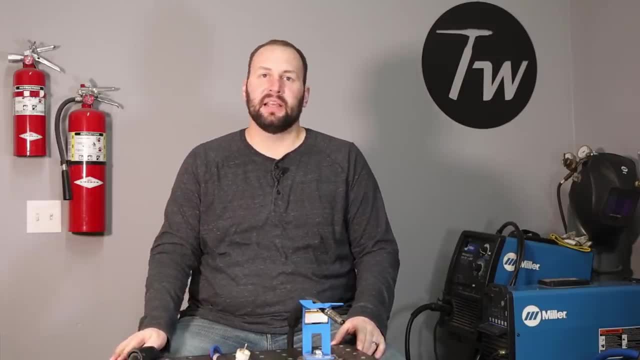 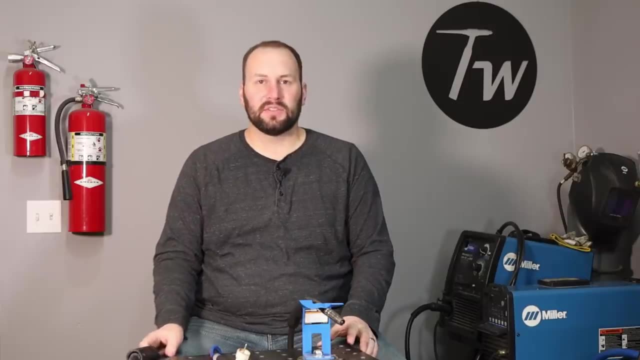 all the way up to this. one's rated for three sixteenths of an inch, But there are industrial processes that weld extremely thick things, You know, using heavier duty equipment with flux core process. So so it's good for for all of that. 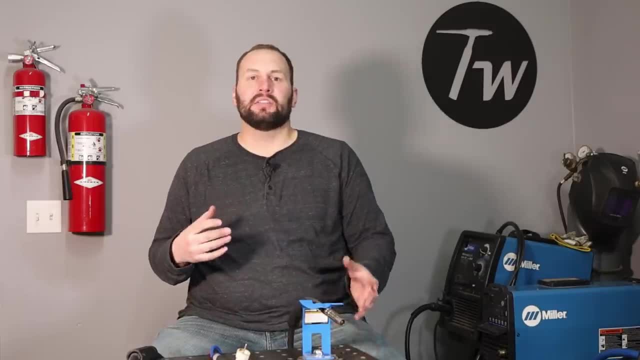 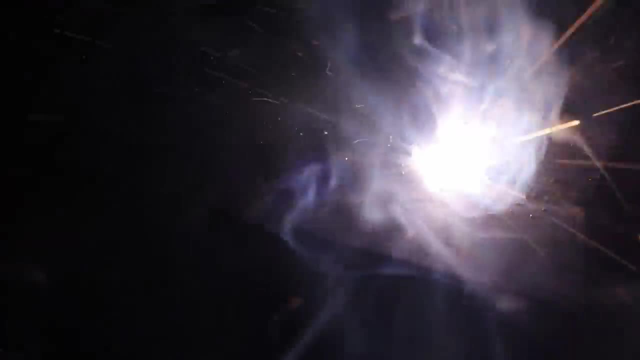 You still still have that slag to deal with, right? So watch as I weld along here. You can see. I'm just maintaining a steady distance with my arc between the end of the gun and the work piece and moving along, And it's depositing metal in just the same. 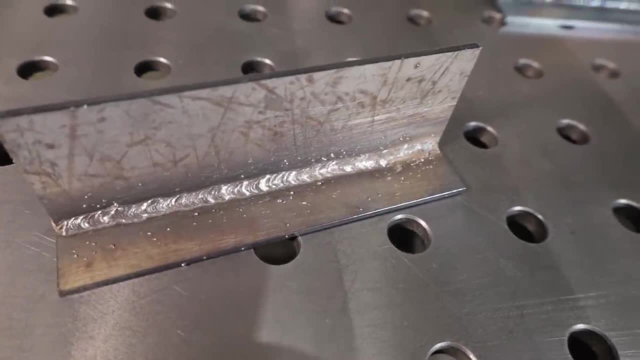 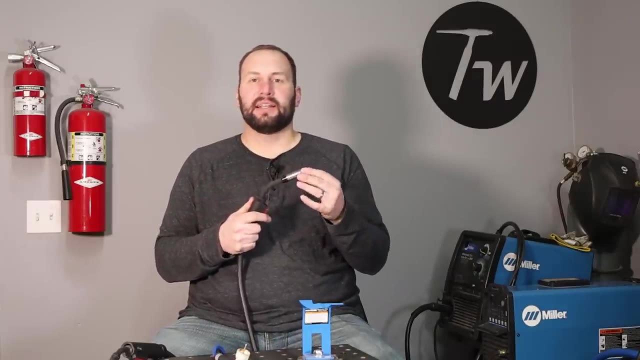 And at the end, after I remove my slag, I got a pretty nice result. Now let's move on to MIG welding. This is the process I use the most in my shop, because it's fast to run. It doesn't leave any slag coating. 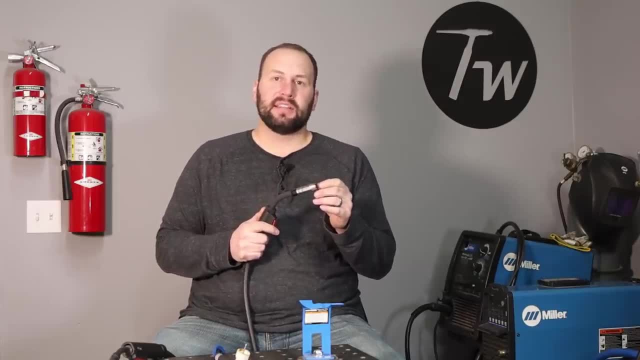 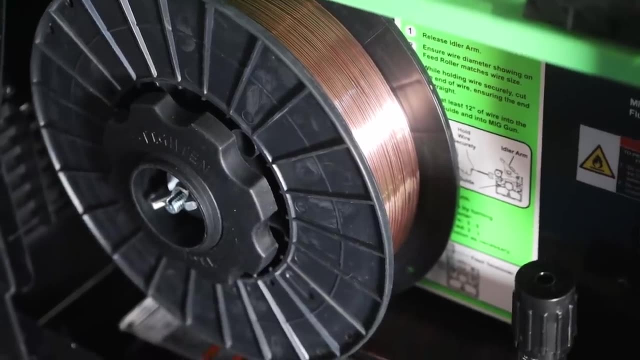 And the reason for that is it doesn't use a flux. So let's look at the equipment here. You can see that there's this roll of wire and it looks like copper wire, but it's actually steel wire coated in copper to protect it. 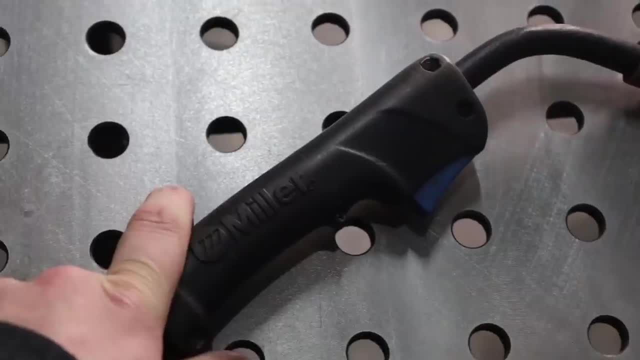 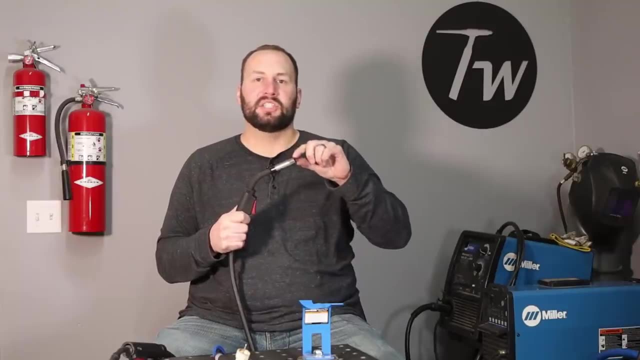 And that wire gets fed through and out of gun the same way as with the flux core welding, except this time there's a nozzle around the outside And shielding gas which comes out of a gas cylinder, and that's either carbon dioxide or argon or a mixture of the two. 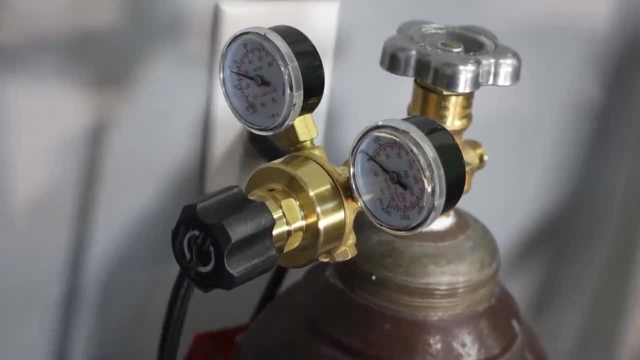 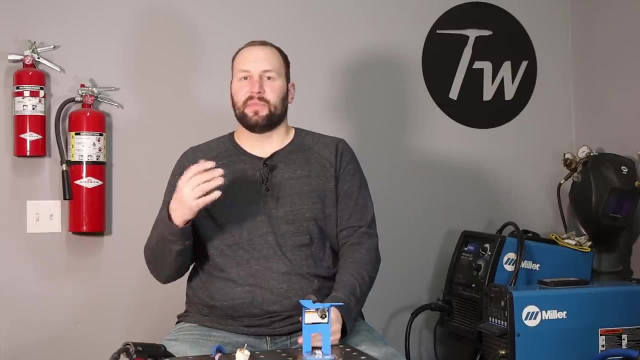 Most of the time, that gas will protect the weld pool instead. That's nice because you don't get the slag. So it's really good for anything from thin sheet metal. It's great for auto body work. It's great for all sorts of things. 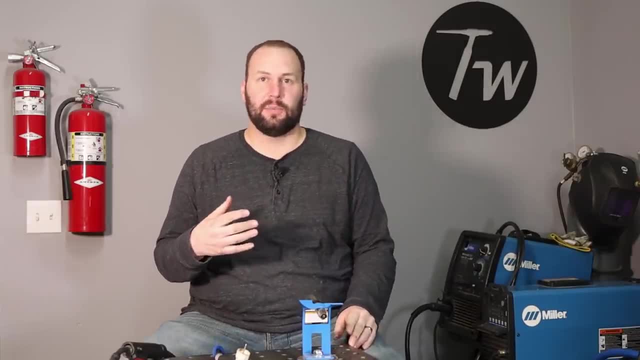 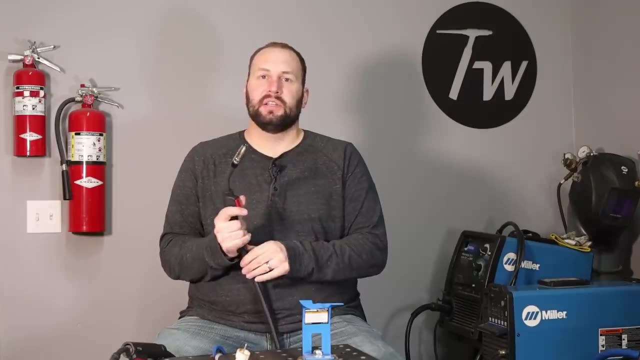 Clear up. my machines will run three eighths of an inch thick material in a single pass, running on 240 volts. So that's with a relatively small machine. So so it's good for for many, many things. You can see as I weld along here. I'm just, you know, doing a small. 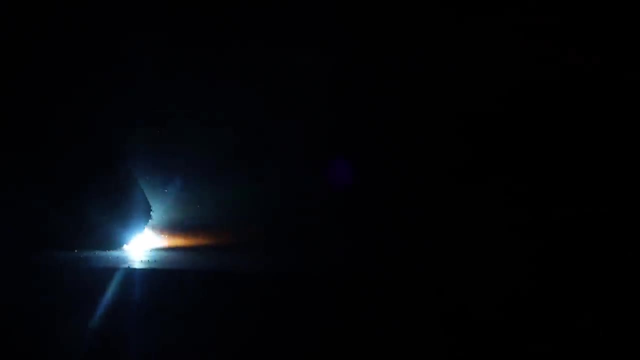 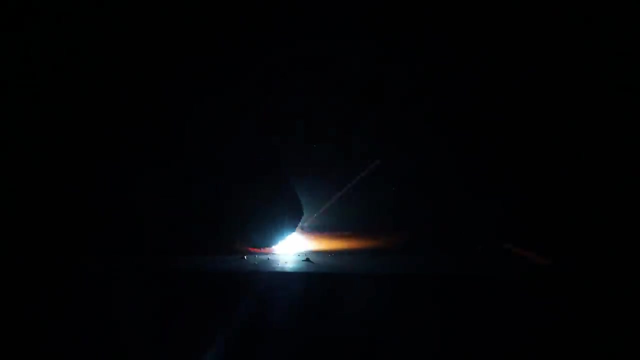 oscillating motion and it's filling in that weld. But I don't have that slag on the top And so after I'm done it's just really nice and clear and clean. Now one of the drawbacks to MIG welding is it'll be more expensive. 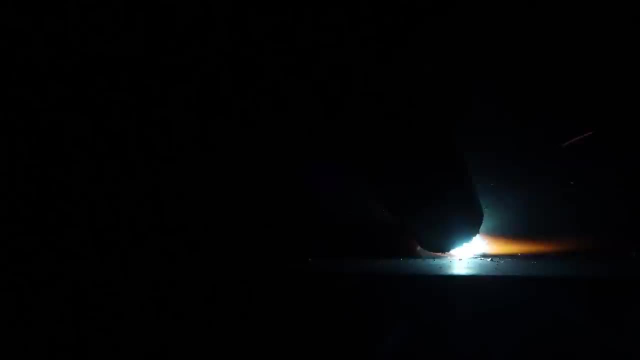 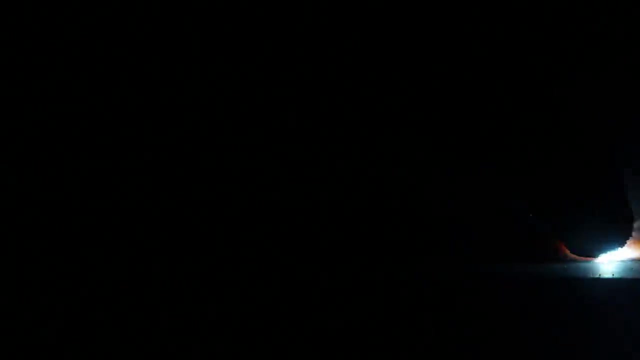 than either flux core or stick welding for the equipment, because, One, the machines are typically a little more expensive And, two, you need that gas cylinder to go along with it. So keep that in mind when you're making your decision. But, like I mentioned before, 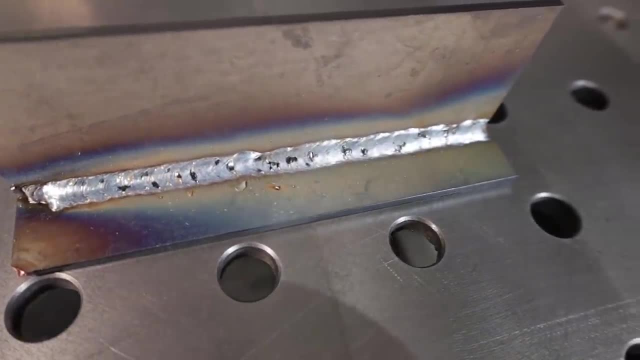 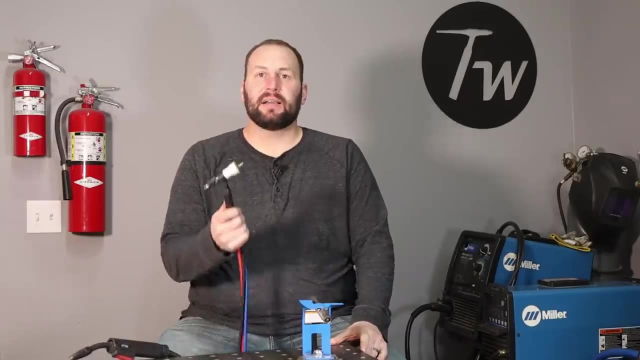 you can start out with just the machine and run it on flux core wire and then get the gas cylinder at some point when you want to. It's also less portable because you need to take that gas cylinder with you. Finally, let's talk about TIG welding or gas tungsten arc welding. 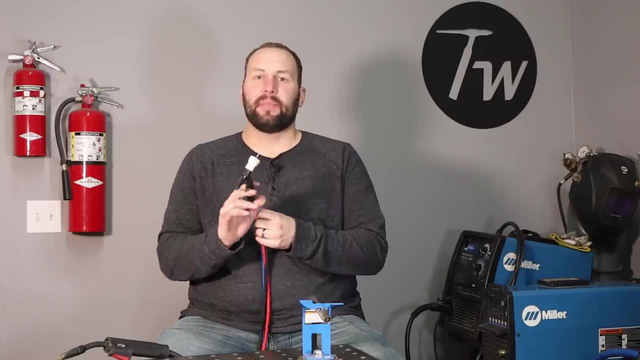 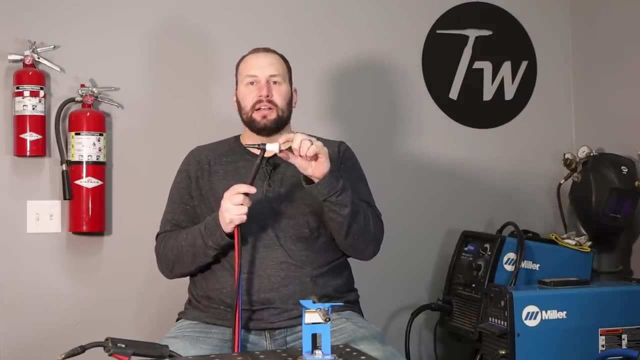 It's often called- And imagine- the MIG gun that we had before, because it has the gas nozzle that comes around the outside, But instead of wire feeding out through the center, just put an electrode that won't melt, And this is made out of tungsten alloy. 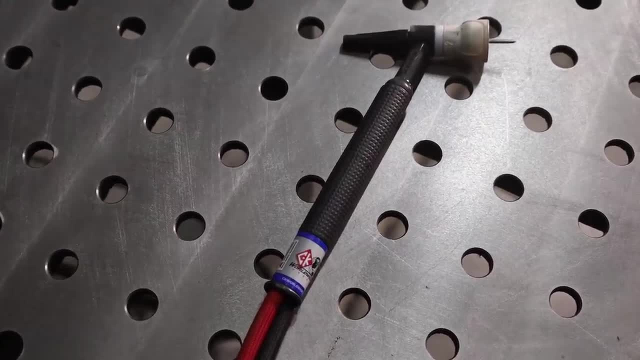 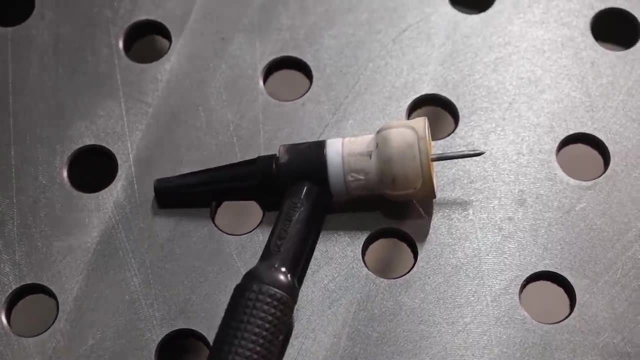 And it's similar to you know, in a light bulb you'll have a tungsten filament, because it can get hot and not melt in an old fashioned light bulb, And so you can create that arc and concentrate the heat there and you decouple that from adding metal to it. 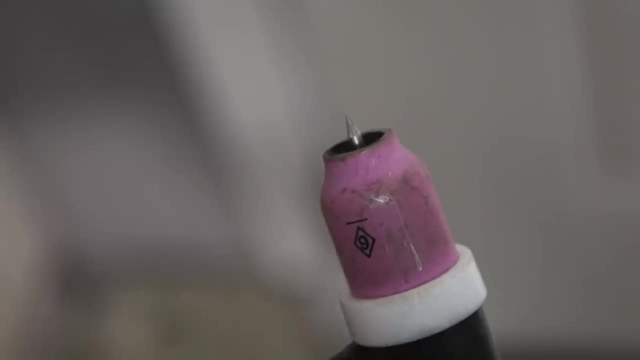 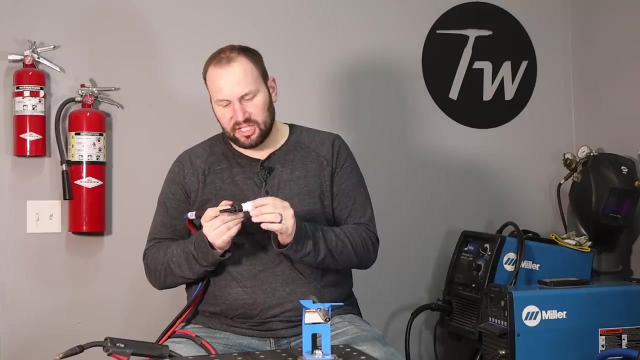 And so that makes it work really well for precise work where you want to have Really fine control. So it's the most well controlled and precise of the processes, though the most challenging to learn. So in order to add that filler metal, you just use an additional rod. 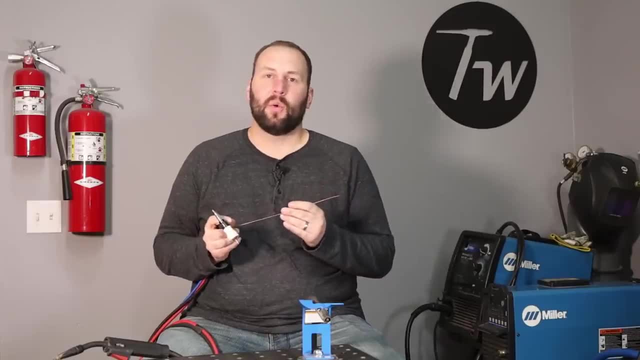 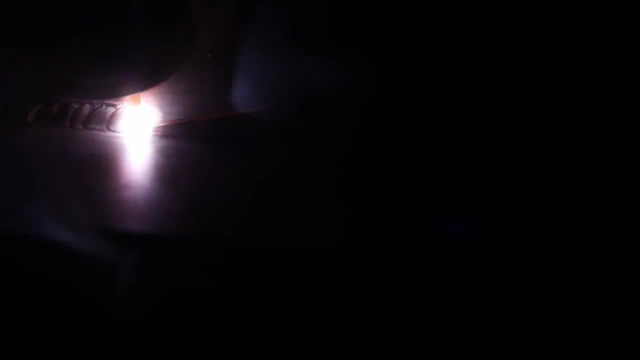 and you'll feed that right into your weld pool. So watch as I run this here. I'm just creating that weld pool And as I move along I'm just adding that filler metal right to the leading edge of the weld pool. here on this steel weld coupon. 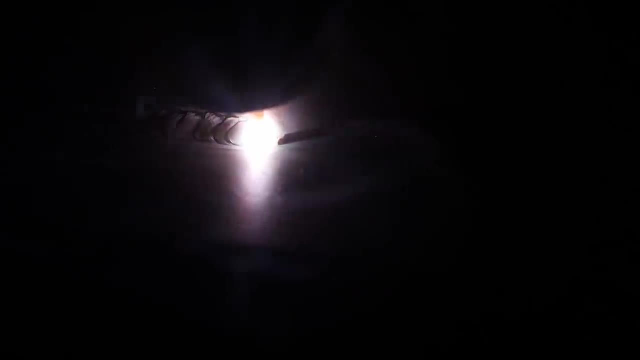 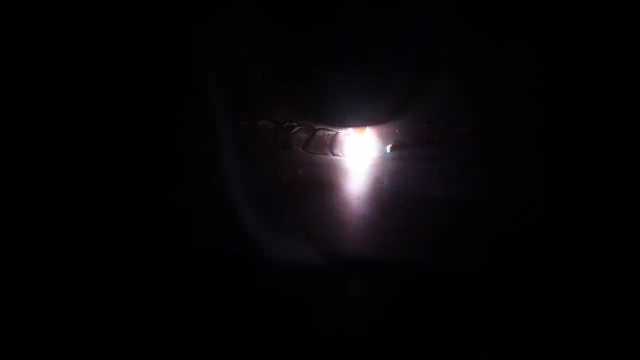 And you can use TIG welding for aluminum. It's the ideal process for welding aluminum, but you will need to get a machine that will output alternating current or AC as well as DC, and that will increase the cost of the machine. So, as far as cost goes, there's a gas cylinder similar to MIG welding. and TIG welding machines are, you know, in a similar price range to MIG welding machines, with the alternating current options being on the higher end of it. So you know you're fairly similar there in terms of price for the machines and portability. 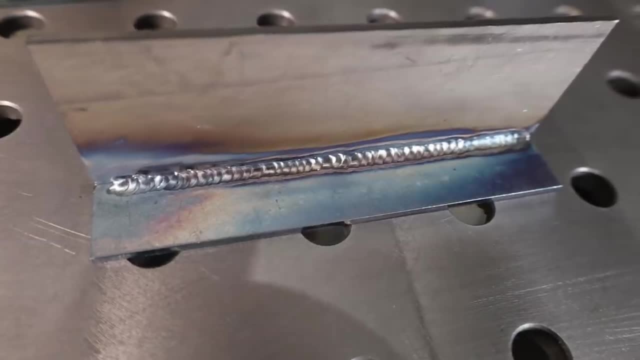 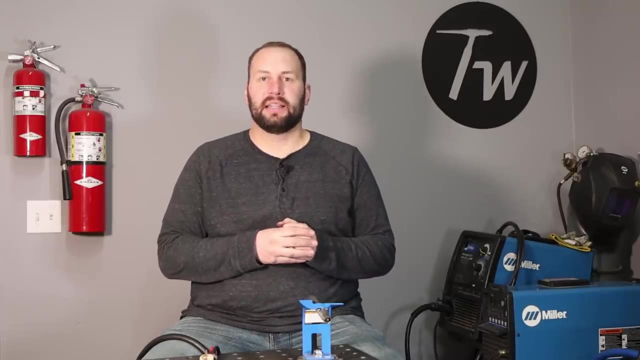 One thing to keep in mind is almost all TIG welding machines can be used to stick weld, So I've taken my TIG welder before and just used it for a stick welding job. So that is an option for you if you get that.